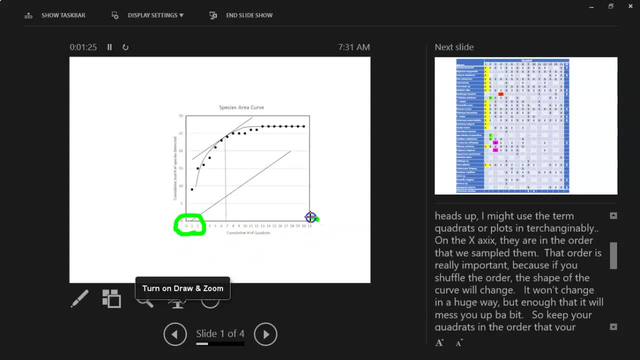 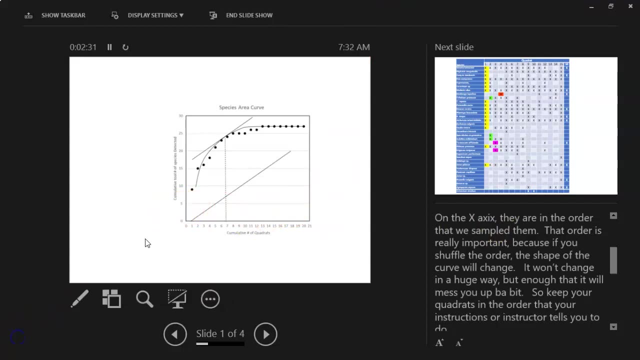 this particular study, This quadrat over here, number 21,. this was the very last of the quadrats sampled. That's a lot of quadrats. I'm sure they were tired by that time. Okay, moving on, let's look now at the y-axis. Actually, before I move, 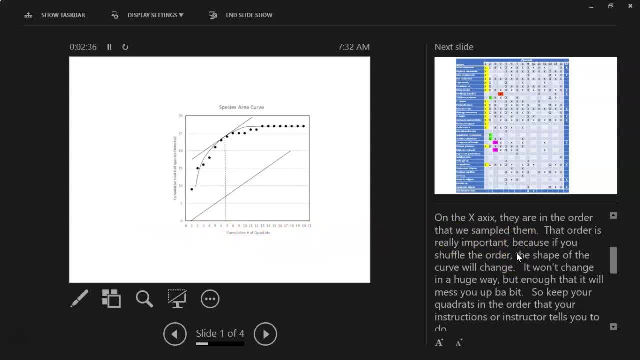 on to the y-axis, I realized that I need to point out that it's really important to keep the quadrats in the order that they were sampled on the x-axis. That order is really important because if you shuffle it, the shape of the curve is going to. 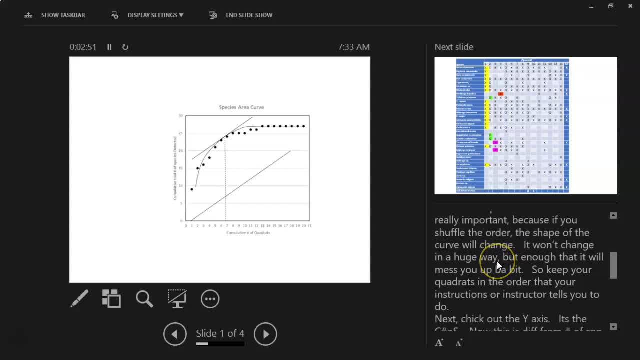 change. It probably won't change the outcome in a huge way, but it'll change it enough that it'll mess you up a bit And what you would wind up is something different than the person grading your lab work would get. so you'd lose some. 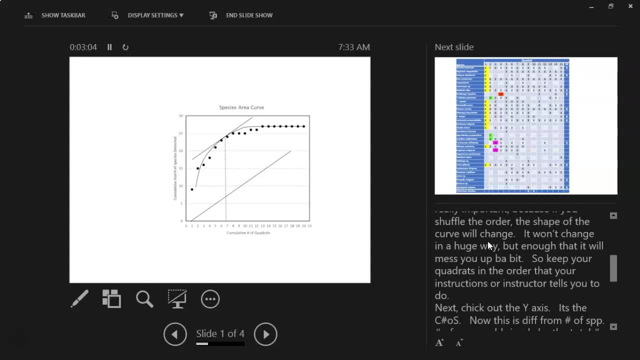 points there, for sure. Okay, so keep your quadrats in the order that your instructors, or that your instructions, tell you to keep, in the order that they were sampled. Okay, now let's look at the y-axis. What the y-axis is showing is the cumulative number. 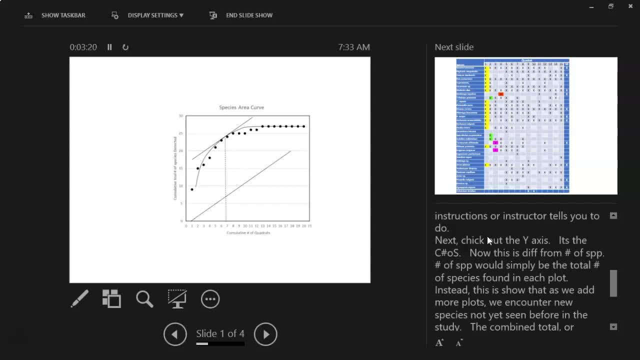 of species. Now, this is different from simply plotting the number of species in a quadrat. That would be simply the total number of species found in a quadrat. Instead, this is showing that as we add more plots, we encounter new species not yet seen before during the study. 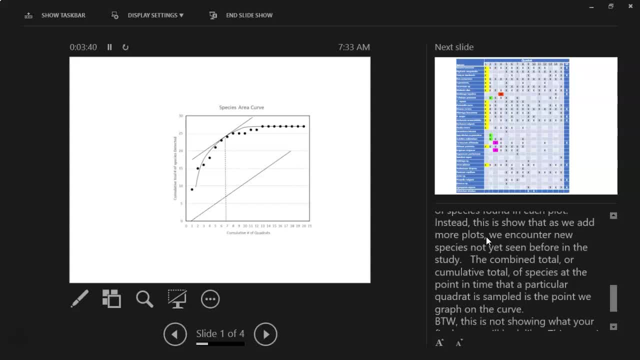 And the combined total of species or the cumulative total of species at the point in time that a particular quadrat is sampled is the point that we graph on the curve. Now, if that seems still confusing, don't worry, I'm going to show. 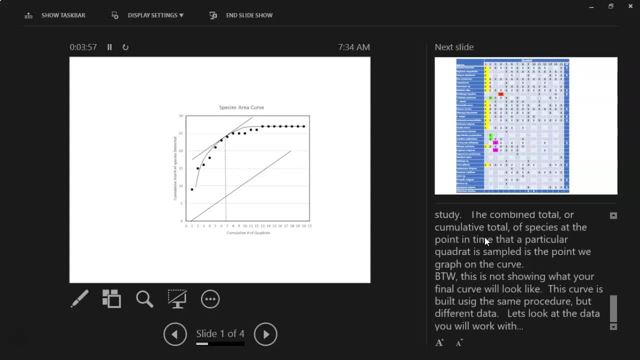 you how to do that in just a minute. And before I get into showing you how we do that, let me point out that this is just a sample species area curve that you're looking at here. It's built using the same procedure, but 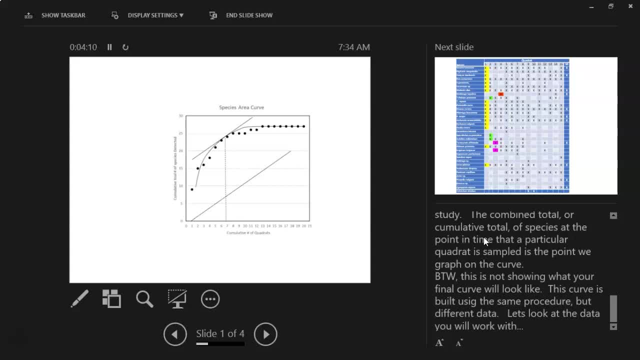 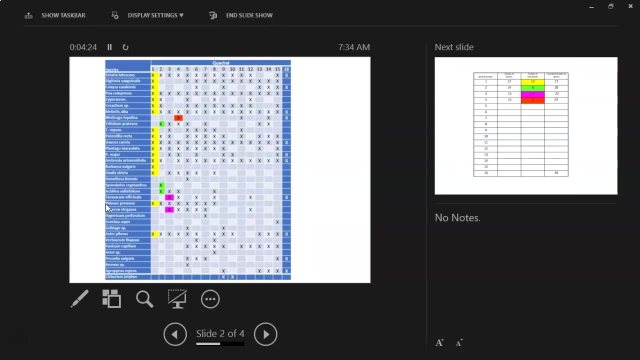 with different data that you're going to use in your lab. Okay, so now let's look at the data that you will work with in the Lab 2, the ecological sampling simulation. Okay, these are the data that you're going to see in your lab handout. The colors are different because I'm working through PowerPoint. 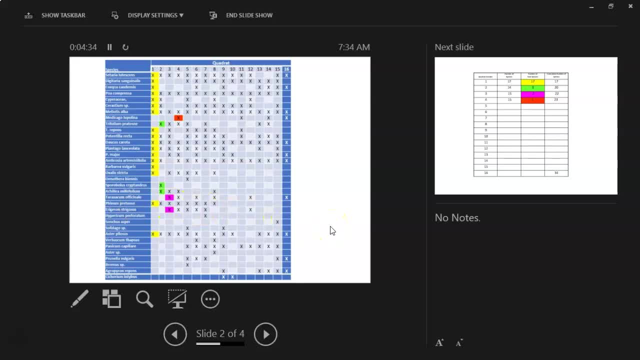 and not through a doc file in your lab notebook or in your lab handout. What we're looking at here is the results of a study done looking at plant species in 16 quadrats in a field up in the Midwest. The first thing I want you 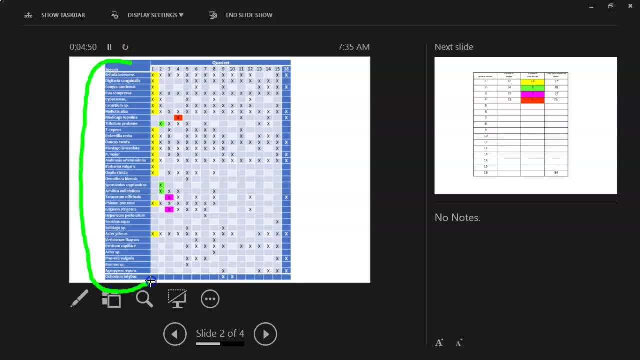 to note is that these are the species that were found during the study that I'm circling here on the left And then across the top. these numbers that are up here- 1 through 16, represent the 16 quadrats that were sampled in this study. 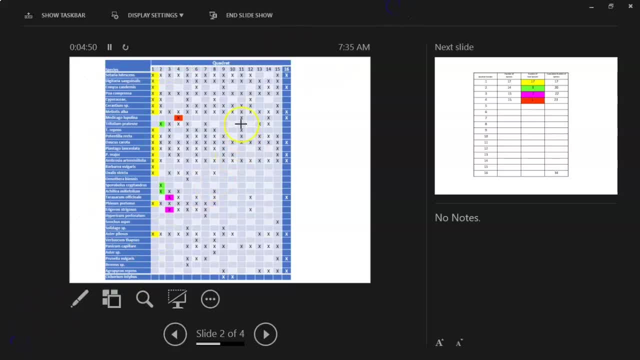 In the body of the table you see a bunch of X's. An X indicates that a particular species was found in a particular plot. So, for example, this X right here represents that the species Taxicum officinale was found in quadrat number 12.. Okay, you'll also see that it was found. 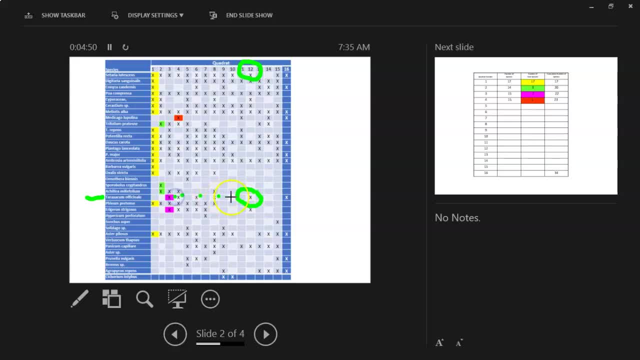 in other plots. This is indicating by these little green dots here, but this cell right here tells us that that species was found in that particular quadrat. Okay, now to graph a species accumulation curve, a species area curve. I should say you need to organize these data that you're looking at here in a special format. So let's. 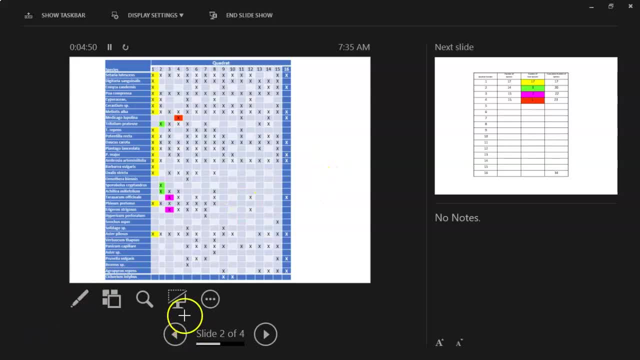 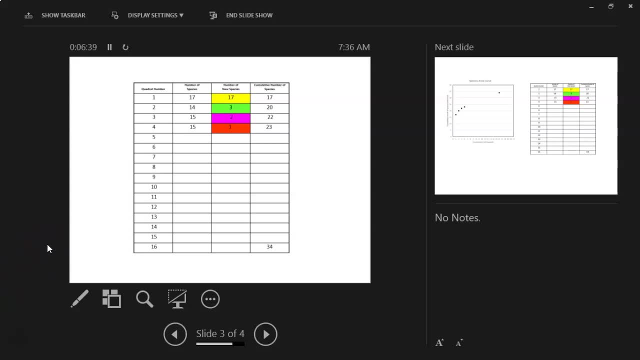 take a look at that. Here's an example of the way that you need to organize those data from the previous table that I showed you in a way that you can graph the cumulative number of species. So what I want you to notice here is that you've got your quadrats in the far left, column 1, through. 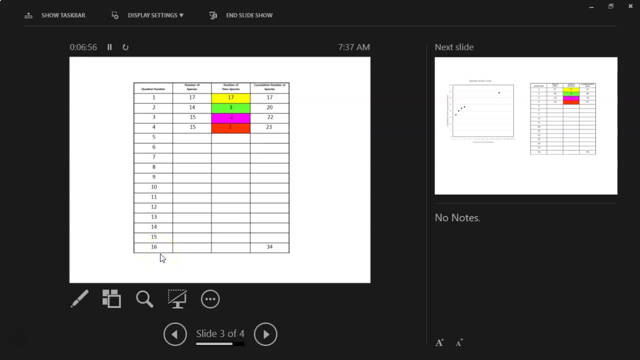 16,, just like we saw before, And they're in the same order as before. And then across the top we've got four different categories of number. We got quadrat number. We've got of species in the quadrat. We've got number of new species for the study that were detected. 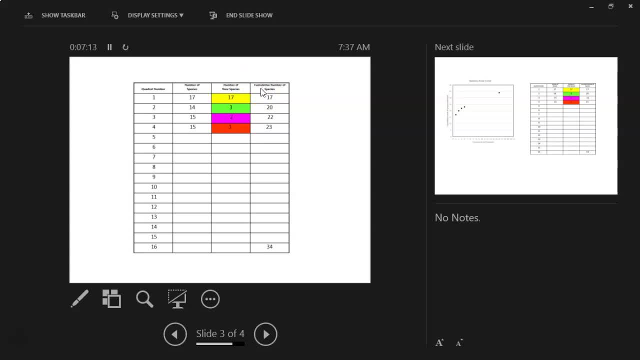 in that quadrat And then we have the total cumulative number of species seen in the study so far when that quadrat was done. So let me show you how that's conducted. By the way, these colors here are going to correspond to the colors in the previous graph. 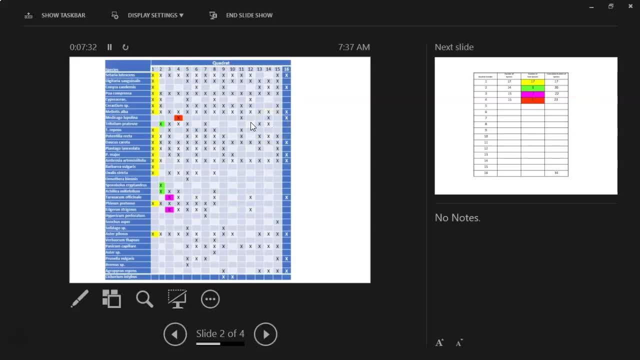 Okay, so now we're back at this chart that shows the raw data. Let's look at quadrat number one. The x's here that are highlighted in yellow are all the x's indicating all the species that were found in quadrat number one. If you were to count them up, you would find that there's a total of 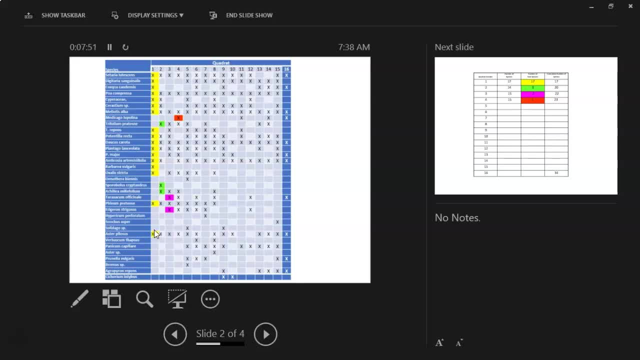 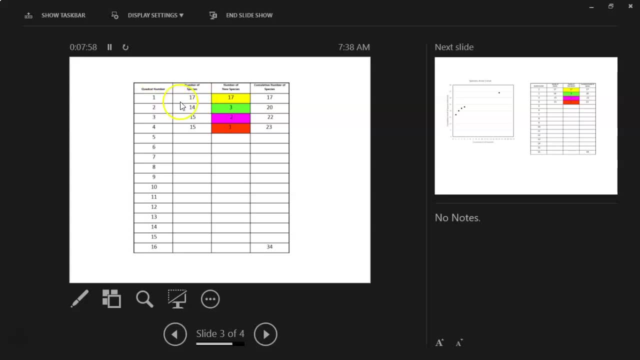 17 x's in that column. So 17 is the number that we would put here and the number of species found for quadrat number one. Okay now, because quadrat number one was the very first quadrat of this study. all of the species in quadrat one are new species to the study. They've not been seen before. 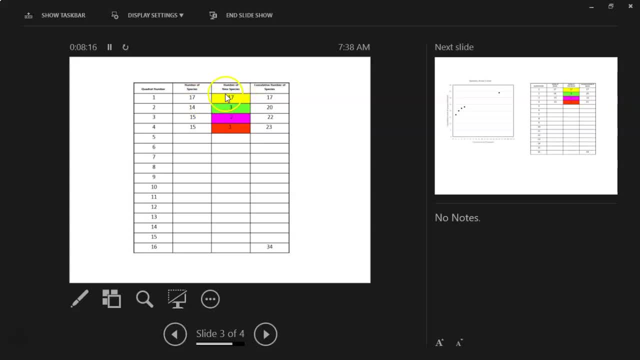 So our number of new species at the point of quadrat one is going to be 17.. By the same logic, the cumulative number of species at this point in the study, at the completion of quadrat one, is also 17.. Okay, let's go back to the table. 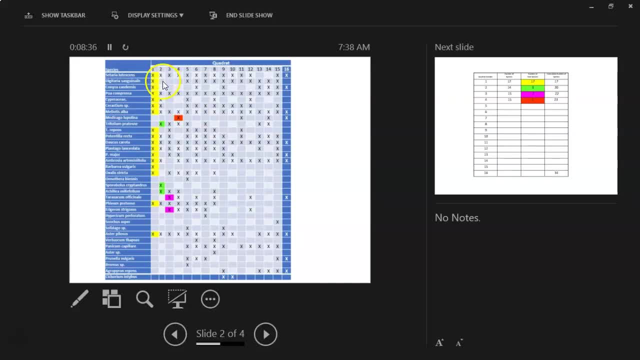 Let's look at quadrat number two. If we look at all the x's in quadrat number two and if we were to tally them up, we would find that there's 14 x's in quadrat 2. And we write that down on our table. Here it is right there. 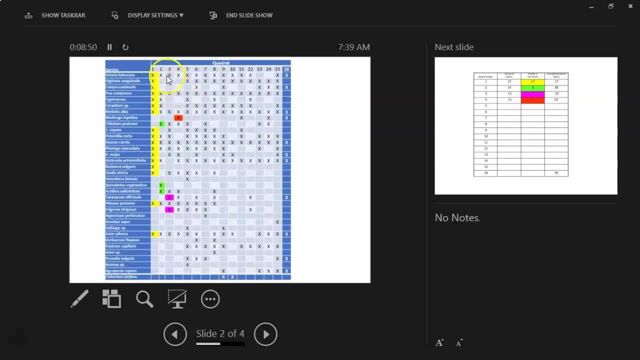 14 species. okay, Now going back to this table, Let's look for species that are new to the study. So as we scan down the table, the column here, we notice that this X here at the very top for Cetaria lutecens, that species was. 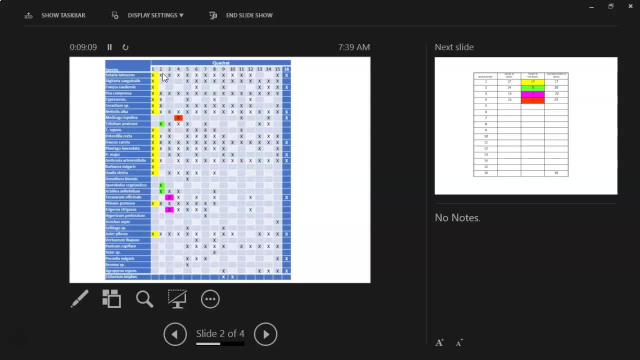 seen in quadrat number one. So therefore this species right here is not a new species for the study, So we're not going to highlight that one. If we were to continue down, we'd find that these four species were also seen in quadrat one, so they are also not new. But when we get to here, 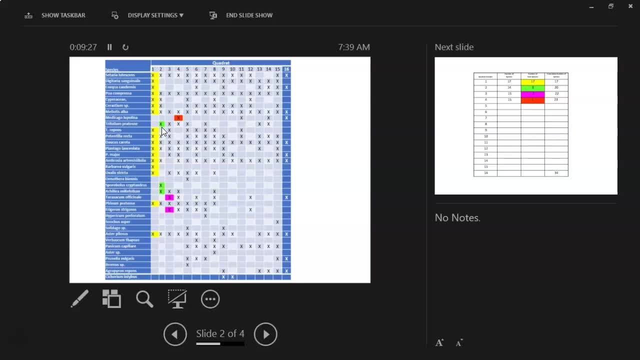 with this cell that's highlighted in green. we do have a species that's new. This is Trifolium pretensis- or- I can't read it, let's see Pretesni- And this species was not seen in quadrat number. 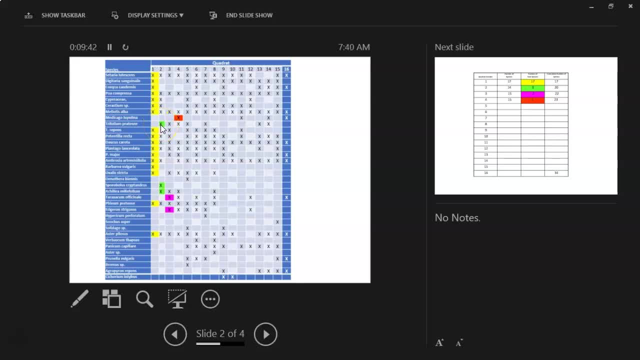 one. So we're going to highlight that here because we're going to have to count up the species that are new to the study, that we hadn't seen in previous quadrats. Scanning on down here we see a bunch that had been seen in quadrat one. We get to two more that are brand new. 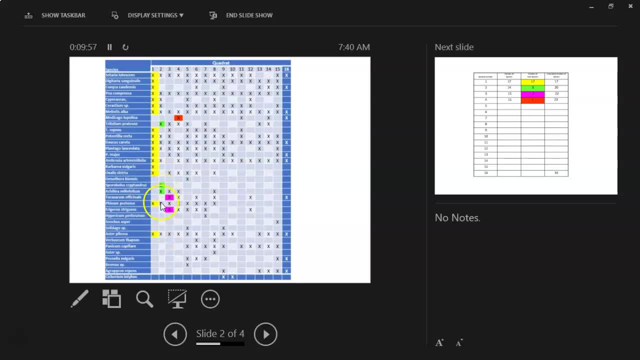 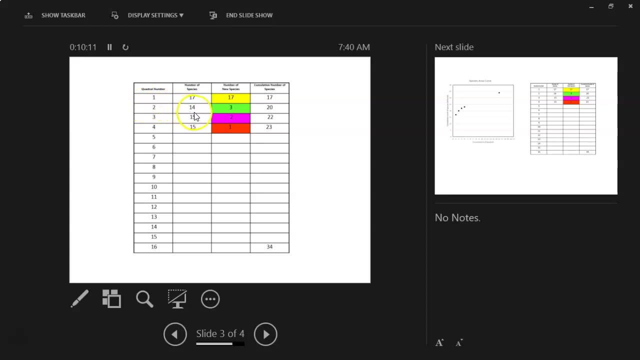 and in quadrat number two. And it turns out that these three that I've highlighted in green are the only new species added to the study that were detected in quadrat two. So let's look at our table and how we organized that. So here we go. quadrat number two: Our total number of species. 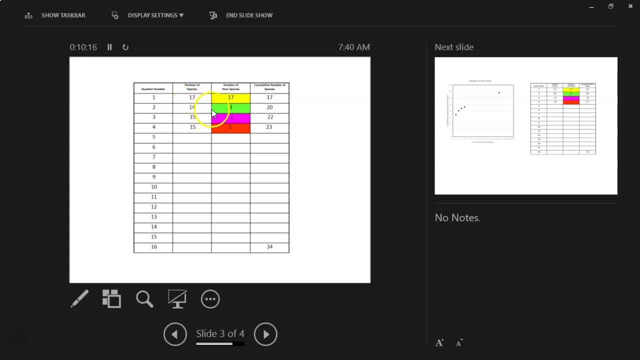 was 14.. There were 14 X's in that column. The number of new species contributed to the study by quadrat number two was three. Those were those three species that were detected in quadrat two. These are the species I highlighted with the green on the previous chart. Now our cumulative number. 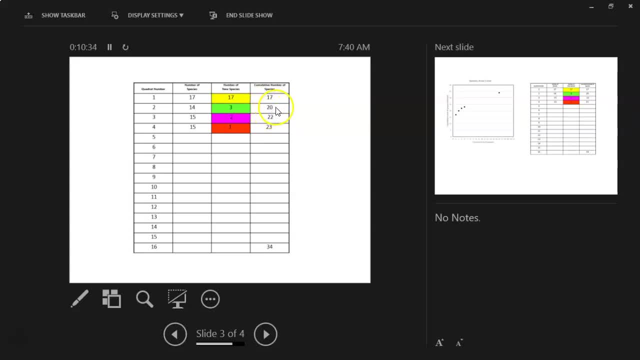 of species and this is the number that you're going to be graphing. our cumulative number species now is at 20.. We had the 17 new species from before plus the three species that were new to the study. in quadrat number two, 17 plus 3 is equal to 20.. Okay, so far looks so good. Let's do a. 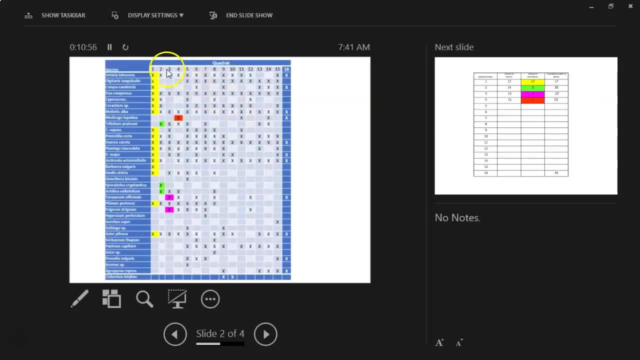 couple more of these, so you get the hang of it In quadrat number three. if we scan through the column we find that all of the species in quadrat number three- so far until we get to down here, were all seen in the previous quadrats. But these 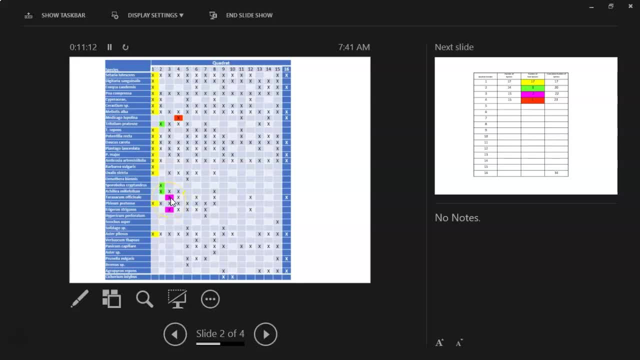 two: this species right here and Erigeron's Trigosis. these two species highlighted in purple are brand new to the study. They were not seen in quadrats one or two. You can see that those cells are empty. So we're going to go ahead and look at them. So we're going to go ahead and 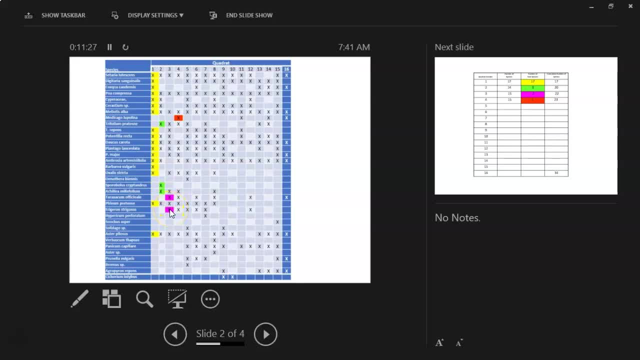 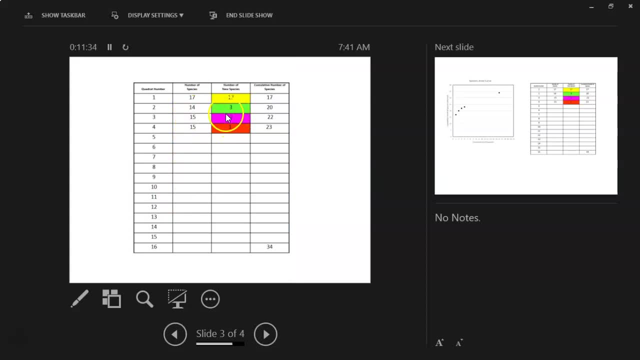 look at them. So we've got a total of 15 species in quadrat number three. So we write down 15. here We've got our two species that are new to the study and then our cumulative number of new species would be the 20 cumulative species at the end of sampling quadrat two plus the two new. 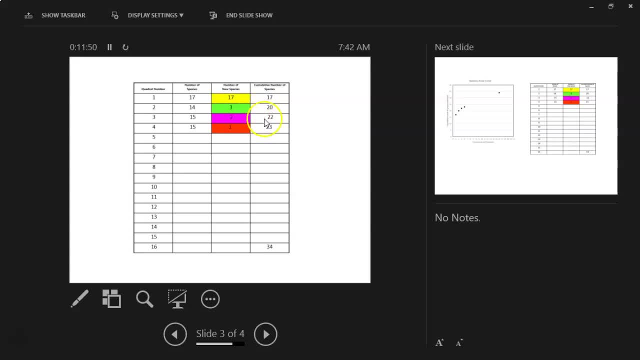 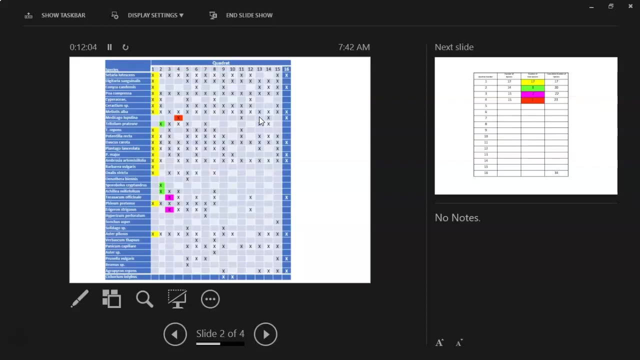 species that we have at the end of sampling quadrat three, and that yields a total of 22 new species- I'm sorry, 22 cumulative species in the study thus far, by the time you're done sampling quadrat number three. Okay, one more, even though you've probably gotten the hang of this In quadrat number four. 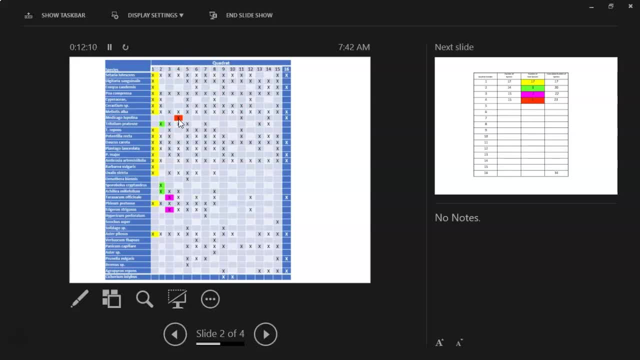 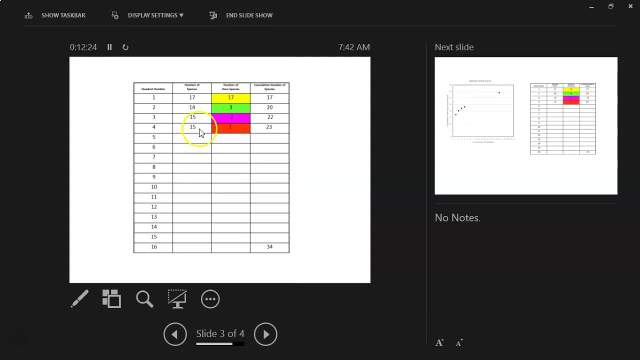 there's only one species that is brand new to the study. All the other x's in column four represent species that had been seen in one of the previous quadrats. So there's a total of 15 species in quadrat. So we write 15. here. There's the one species that was new to the study, And so now our cumulative number of new. 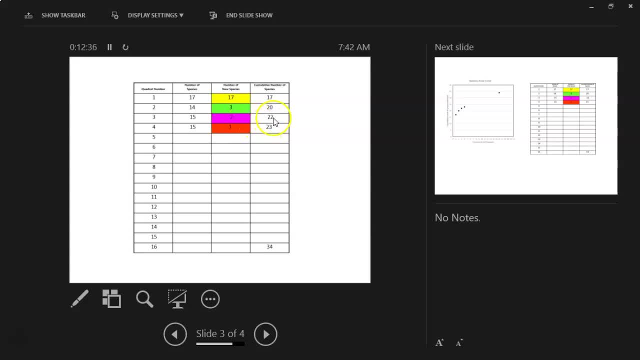 species is 23.. That's the 22 here plus one, is equal to 23.. Okay, now you're going to in lab, the lab for the ecological sampling simulation. you're going to finish out the rest of this table And we tell you that the total 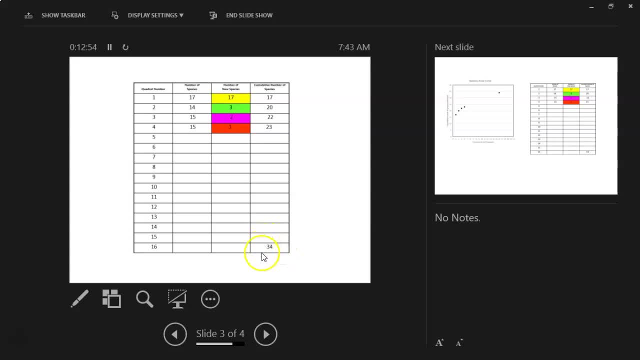 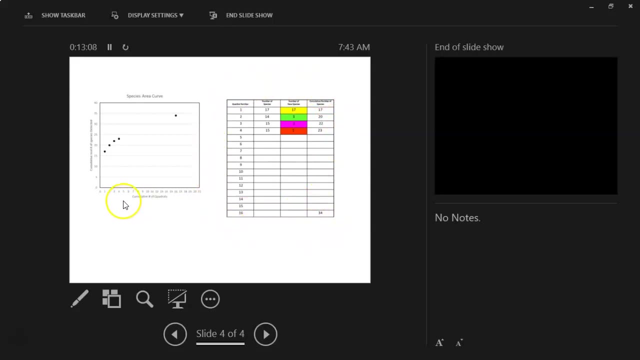 number of species there is 34.. If your number doesn't wind up in the table, you're going to have to finish out the rest of this table. So if you end up at 34 at the end, then you've miscounted somewhere along the way. Let me show you now what it looks like as you begin to plot your data. So here I've got our data tabled on the right and I've got a species area curve that I'm building here to the left. What I want you to notice- and this is important- is that this column here the cumulative number of species. this is what we're graphing. So let's start with this first number here for quadrat one. 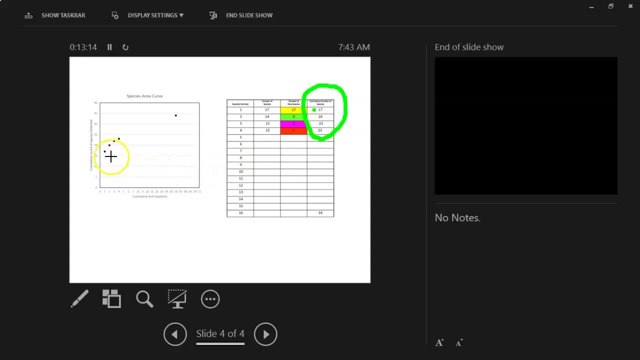 It's 17 new species to the study. That is represented here by that dot, and I'm going to put up my own little green dot right on top of that. Okay, that's 17. if you read it on the y-axis there, The cumulative number of species at quadrat one is at 17.. Okay, for quadrat number two, the cumulative number of species at that point was 20.. So I'm going to plot that right here. This is quadrat number two, Here's 20.. 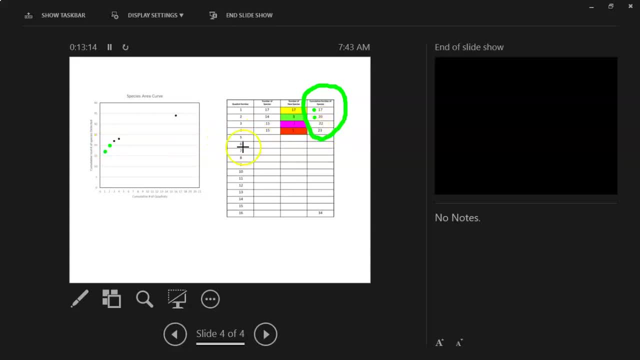 Boom, there's my next dot And then the next two points. you can see where this is going. That would be our 22 for 22 cumulative species for quadrat three, and then 23 cumulative species for quadrat four. Okay, this gets you well on your way to constructing a species area curve. 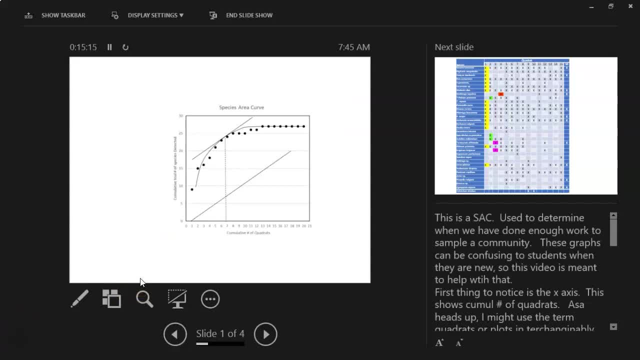 Okay. so the next step, once you've completed your species area curve, is to figure out the point at which it's okay to stop sampling. So I'm going to use this species area curve that's from a different study. It's not the one that is that you will be. these are not the data that you're going to be working with in lab. I wouldn't want to show you how to do that exact lab with this demonstration. I'm showing you here a completed species area curve and I'm going to walk you through how it's done. So first off, note that all the black dots on here 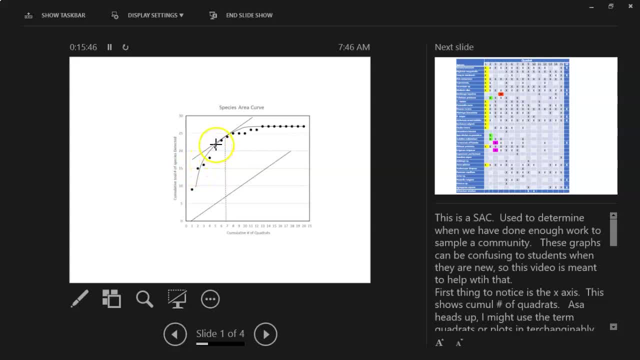 represent the cumulative number of species as you add more quadrats to the study. In this particular study, there were 20 quadrats. Now let me remind you yet one more time that these are not the same data that we were looking looking at in the in the previous graph, because this is just from a different study. Okay, 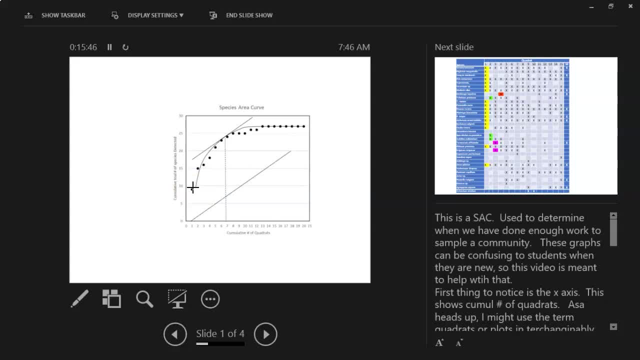 One of the things that I want you to also notice here is that these, as they proceed from quadrat to quadrat, they only go up or over. you never backtrack. you never wind up declining in a number, because this is a cumulative total of species detected as you go up the plot. so it's it almost looks like. 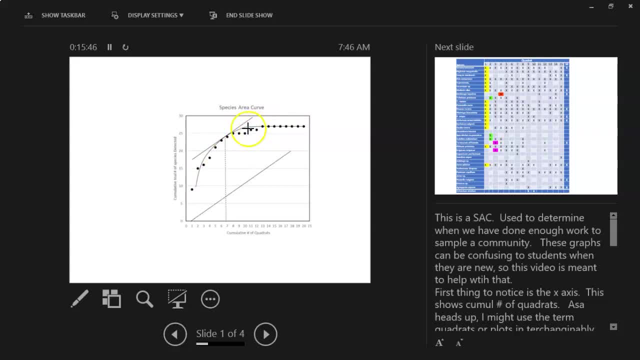 stair steps. if you kind of squint your eyes and look at a little bit, you'll also notice that up here at this part of the graph, that after about quadrat number 12 or 13- I can't really read it carefully- after about this quadrat for. 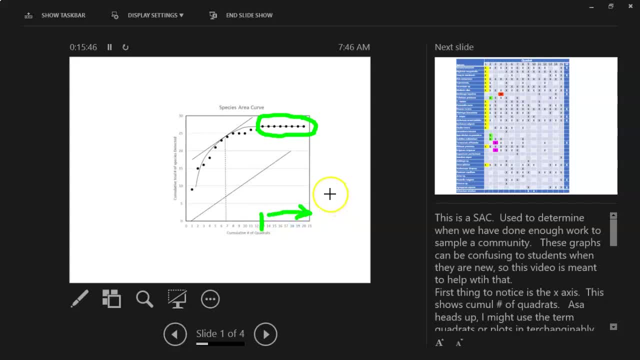 all these quadrats to the right. we did not add any more new species, okay. that's why all all those dots there are in a line, okay, so once you've plotted out your points on your graph, you will then have to do a couple things to figure out. 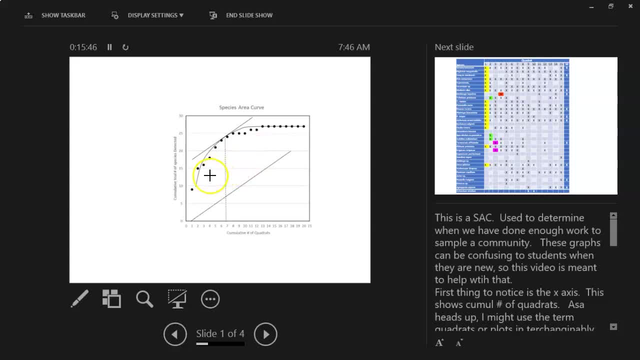 the plot point at which it's okay to stop sampling. the first thing you need to do is to graph a best fit curve, and that's what's represented by this line. that's already on our graph here and I'm going to trace over it using the mouse here. 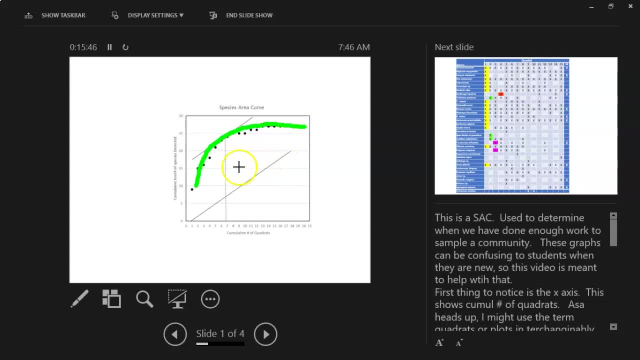 this would be our best fit curve for these points. notice that we're not trying to hit each point. this would not be a best fit curve where you're connecting the dots. okay, connecting the dots is not a best fit curve, so we would not want to do that. so we're going to have to do a couple things to figure out. 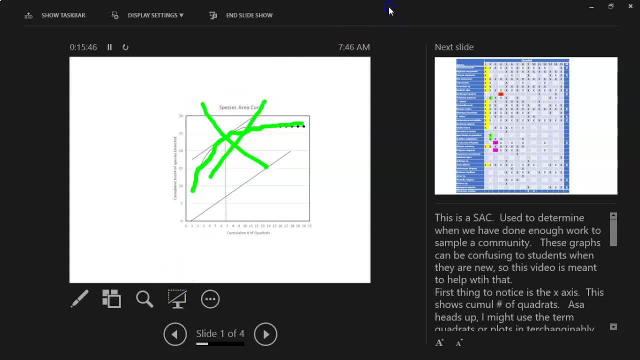 to do that, all right. so this solid black line here that curves up through here is a best fit curve through those points by best fit. you just sort of, as you move through the, the points and along the quadrats, you're, you're sort of averaging out the distances between the points in the line and, quite honestly, this line. 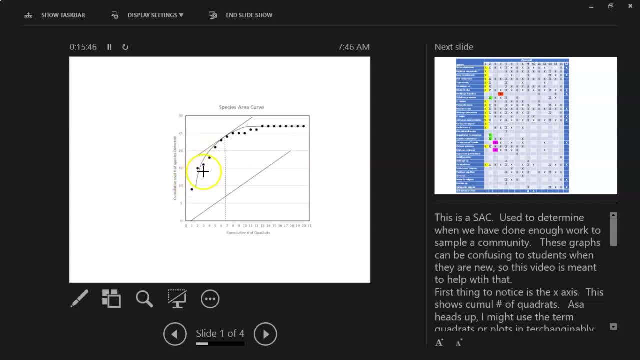 that's already pre-drawn on. this graph could be done a little bit better, but we're going to work with that here. so we're going to work with that here now. we're going to work with that anyway. okay, so we've got our points. we've now. 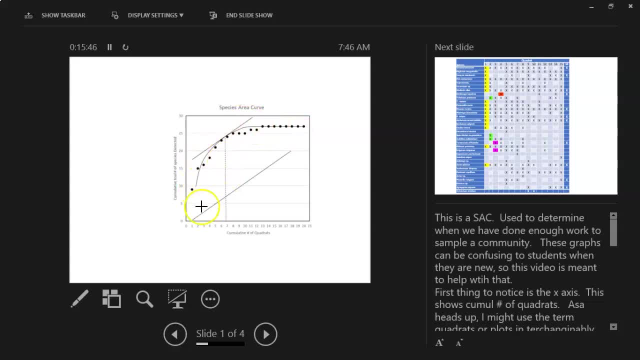 got our best fit. curve these straight lines here. there's three of them: two that are parallel and solid and one that's dotted. those are the things that we're going to do next now to. for this, you need to refer to your instructions about what your goal is for species sampling, and in this case, we want to be. 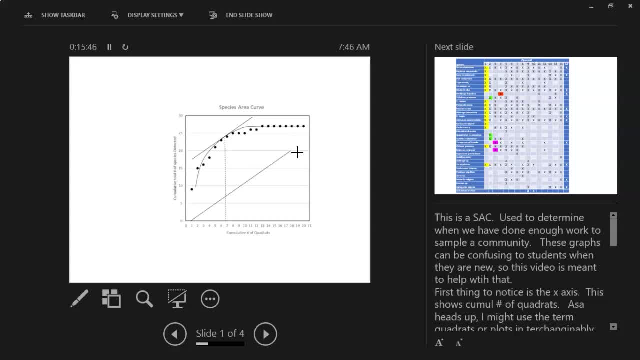 we want to to stop sampling at the point where, when we are adding a quadrat, we are no longer adding a new species of plant on average. okay, so to unpack that a bit, if you look at your species area curve here, notice how steep this part of the line. 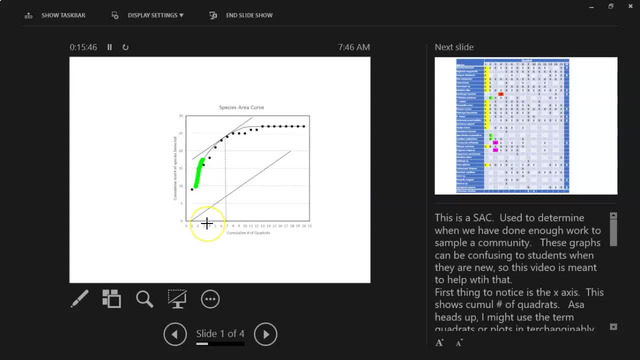 is okay. that's because every time we add a quadrat we are adding, on average, a lot of new species. if we go back to q right here, we are adding the following species: To our first quadrat we added 17 species and then it was three in quadrat two and 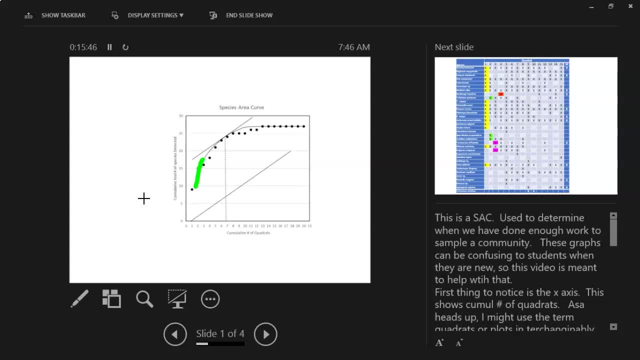 then it was two species in quadrat three and then by the time we got to the fourth quadrat we saw we were adding one species. That's on that data table that we looked at earlier. So for this part of the curve the accumulation of species as we add quadrats is really high. 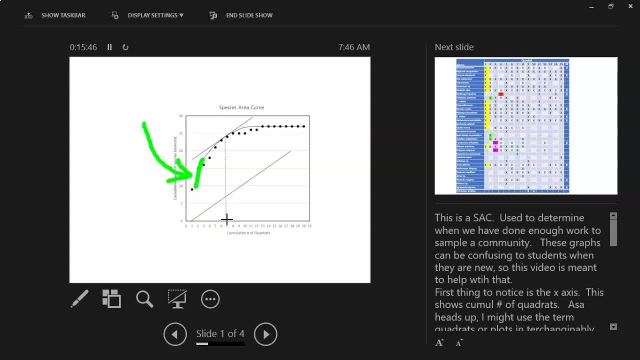 and in general we're adding more than one species every time we add a quadrat. In contrast, on the right-hand part of our curve way over here, every time we're adding a quadrat. sometimes we do not even add one new species. 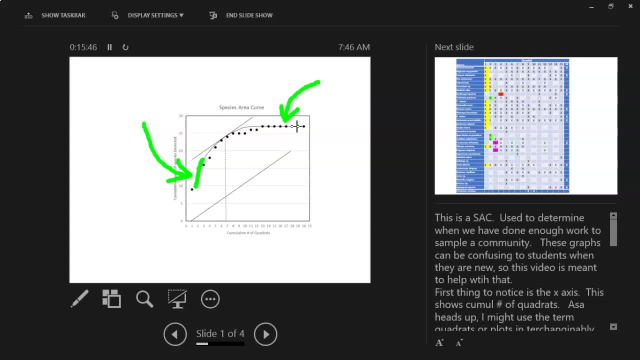 In fact, for this part of the quadrat, our accumulation of new species per quadrat is zero. Over here, on this part, our accumulation of new species is less than one. And because when you consider that you get several quadrats where you don't get any, 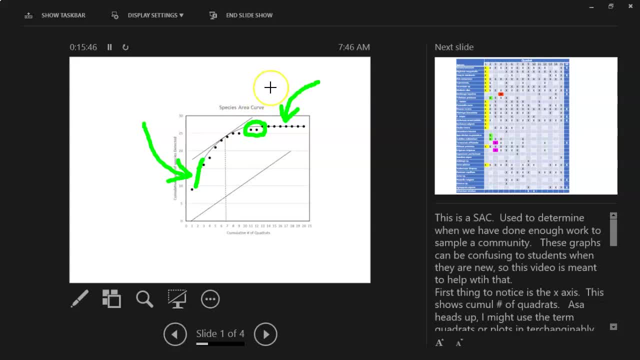 new species. it winds up bringing that average new species per quadrat. it brings that value to be less than one. So it's somewhere right about in here in this part of the species area curve where our rate of accumulation of new species is about at the level of one species for every. 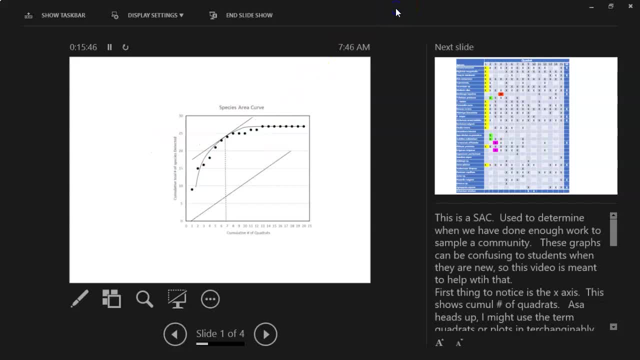 quadrat And we have to figure that out. Okay, so, to figure out where on this curve is the rate we have, the rate of one species per quadrat, we first need a reference line, And that's what this line here- I'm circling the end of it right here- that's what this. 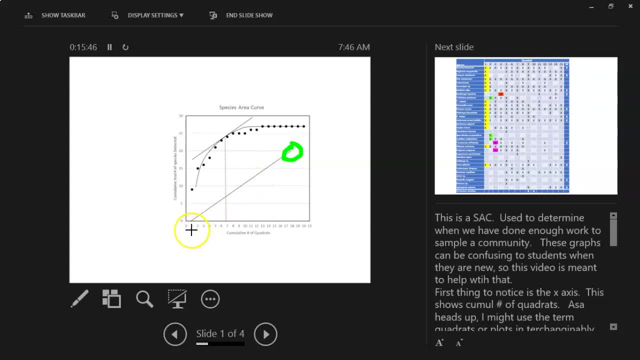 line is all about, And you'll notice that, if you look carefully, you'll notice that what we've done here is that we've plotted it out so that we have a reference line. The reference line shows that for quadrat one we have one species. for quadrat two, 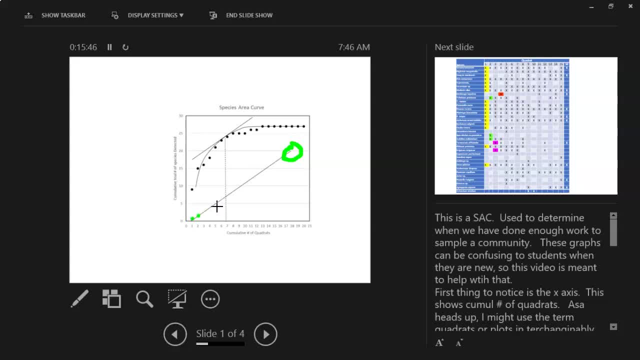 we have two species and so forth and so on. So at five species we've got a five here- I didn't draw that very well- and a five here, And then when we have ten quadrats, here we have ten species. so that's where our point. 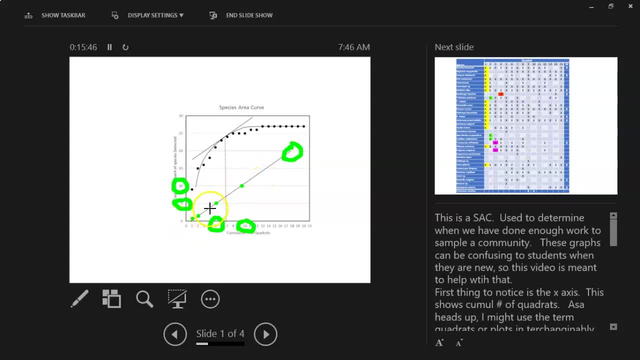 is there and so forth. So, in other words, what this line, this reference line, represents, is what the slope of a curve looks like. I know it's a line, but we call it a curve anyway. But this shows what the slope of a curve looks like when you're adding one species for every. 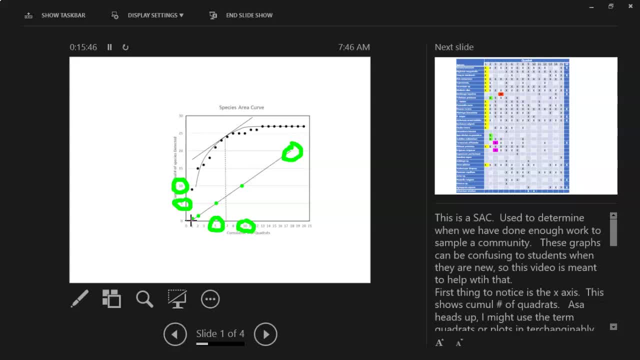 quadrat. Okay, so pause and look at this more carefully, or rewind and look at it again if you need to wrap your head around that, But one more time. this line or this curve is representing the slope at which we're adding one new species every time we add a quadrat. 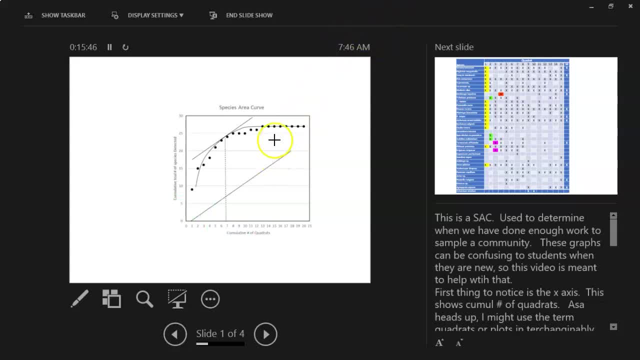 That's going to be our reference line. Okay, the next thing to do is to use this reference line to figure out where we would have a parallel, similar line touching the curve up here at one point. So you'll notice that this line up here, that I'm circling the end of it with a green square. 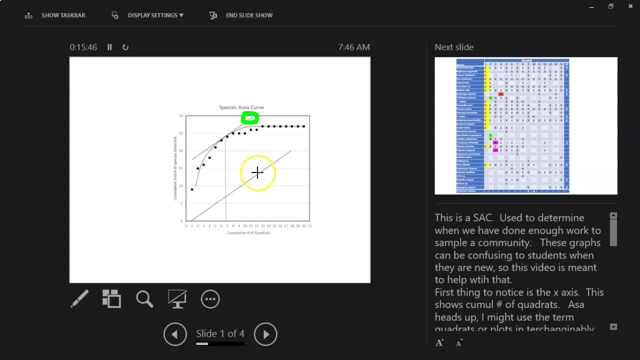 a green circle there. it is parallel to this line. If these two lines were continued on into space, they would never meet, They would never crisscross. either that way or that way. That's what we mean in geometry by lines being parallel. 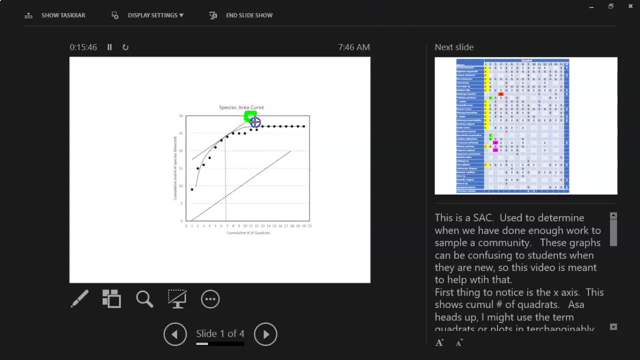 Okay, so we're going to draw this line up here by making sure that it is parallel to this line down here, And you can do that simply by eyeballing it. You can draw a straight edge like a ruler or something like that. 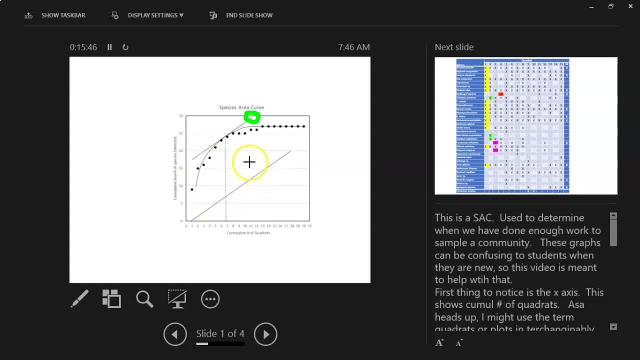 And then holding that straight edge in comparison to this line, you want to make your straight edge parallel and then you draw a line through here where it touches the curve in just one place. Now I realize that it looks like the line is touching the curve in several places, like 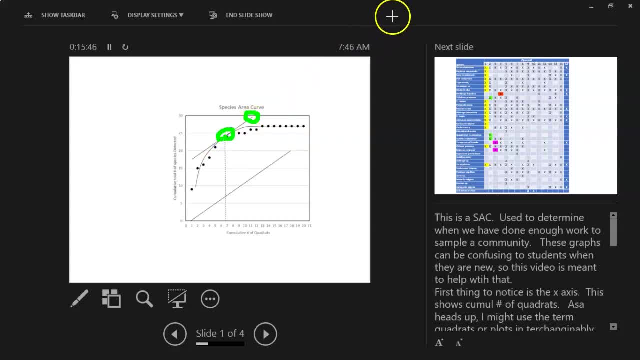 in this whole stretch, right here that I'm circling, But in reality in geometry, in the reality of geometry, it's not, It's not, It's not In geometry. this line is only touching the curve just in one spot, and that happens to. 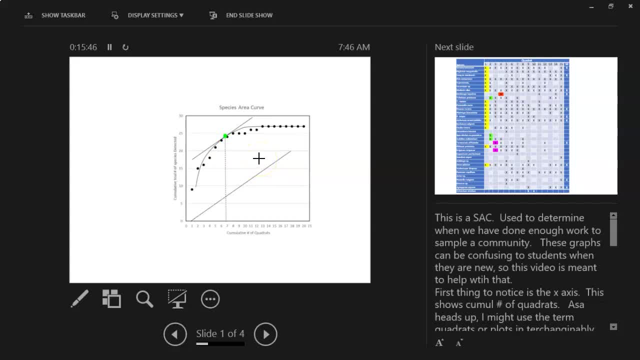 be right about there where I put that green dot. Okay, Even if you can't see it, you can kind of average the distance between where the species accumulation curve and this straight line meet. You know the distance between there and there would be your green dot in the center represented. 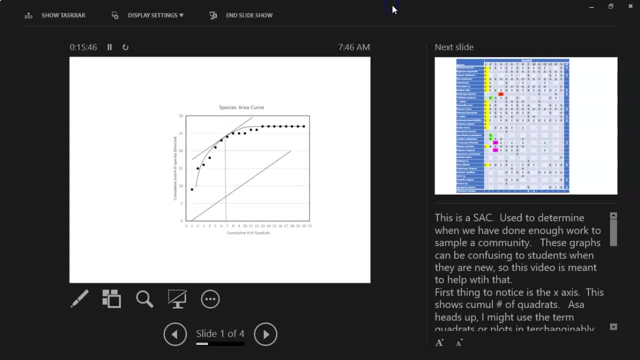 by that big old chunky arrow. Okay, So we now know the point right here where this line is just touching the curve at one point, And that's what we call a tangent line. If it touches it in two points or zero points, it is not a tangent curve. 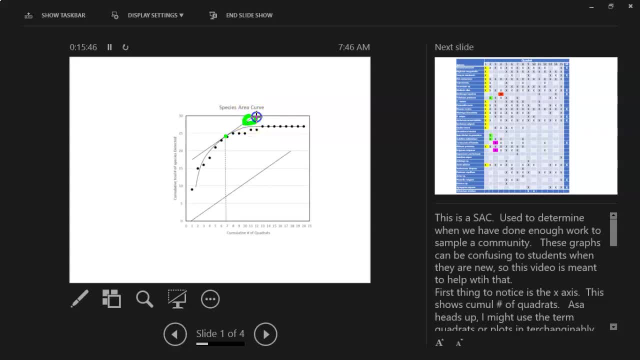 And, of course, this line here, this top line, is parallel to this line, so that we know that where this line is touching our species accumulation curve, That's the point on the species accumulation curve where we are adding one species for every quadrat. 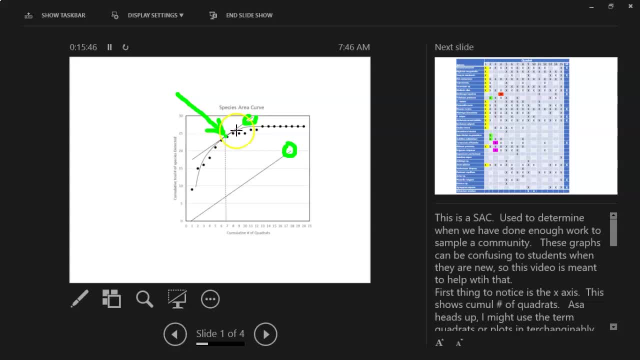 That's the magic point on the curve that we've been looking for this whole time. So the next few steps are pretty easy. All we have to do now is draw a dotted line down from that point, from here straight down to the x-axis, to see where it intercepts the x-axis. 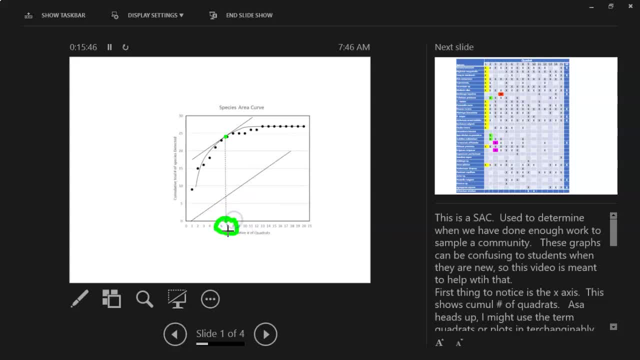 Okay, And that's right about. at seven. Okay, That means that at quadrat number seven is where we had the slope of the slope, representing where we had when we were adding one species for every quadrat To the left of quadrat number seven, we were adding more than one species every time. we 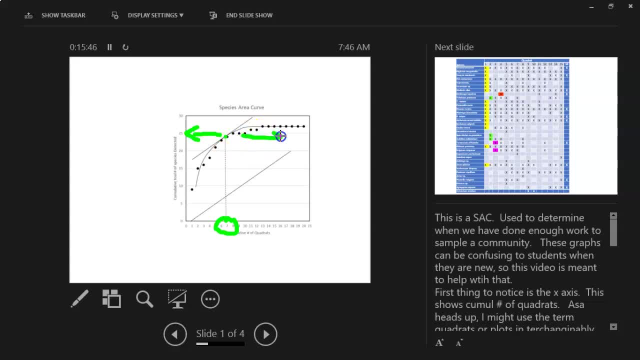 added a quadrat To the right of quadrat seven. we were adding less than one species every time we added a quadrat, So seven is the magic number. Our final answer for where should we stop sampling is quadrat seven. and then we add: 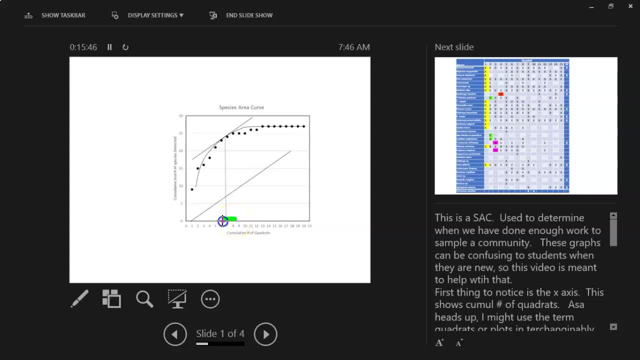 one more sampling quadrat for good measure, just to make sure that our trends are solid. We would stop sampling at eight. So the correct answer in this case would be that sampling should end at eight, which is quadrat seven plus one. Okay, 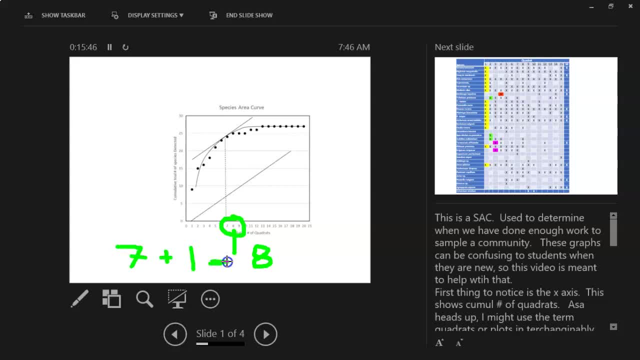 Plus one more for good measure is equal to eight. Okay, So that shows you how to do a species area curve. The instructions are also written out for you in your lab instructions. I hope that was helpful. If not, get in touch with your teaching assistant or your lab instructor.